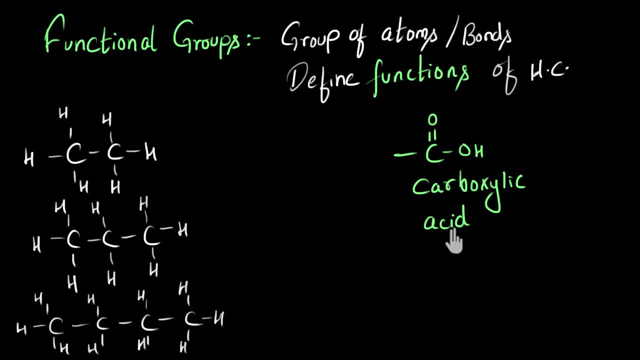 carboxylic acid functional group, and it's called acid because you know the molecule that it gets attached to will now behave like an acid. When that molecule is mixed with water now it will release H plus ions. That's how acids are defined. right Now, let me add this group to a hydrocarbon. 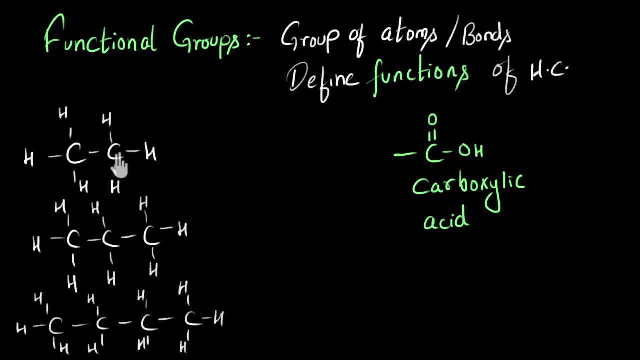 and show you. So, first of all, I'll remove a hydrogen and in place of that I will add this functional group. Now, if you check experimentally, this new molecule will start behaving like an acid When mixed in water. this will give off hydrogen plus ions, H plus ions. Okay, and this: 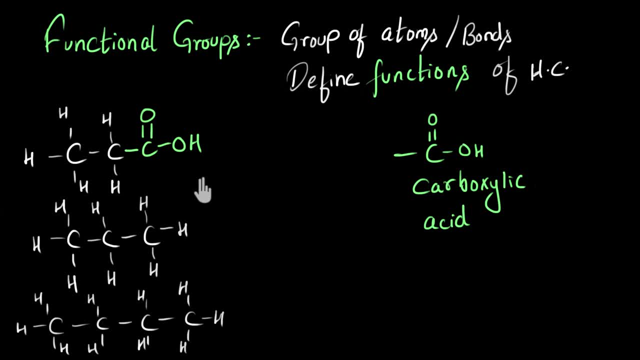 molecule will now have some awesome functions. You can use this in medicine, you can use this in food, you can use this for cleaning purposes, and all of these awesome functions are because of this, This new group of atoms that got added, not this carbon chain. Okay, and if you don't believe me, 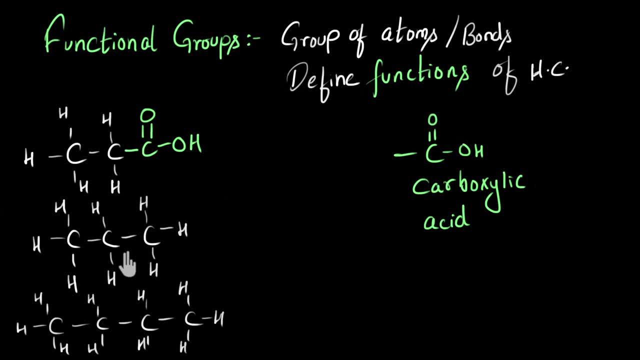 let me actually add this group to a different carbon chain. Here we have three carbons. right Now I can replace a hydrogen atom with the functional group. Now this molecule also will have similar functions like an acid, just like this one. Okay, now let's do it for another carbon chain. 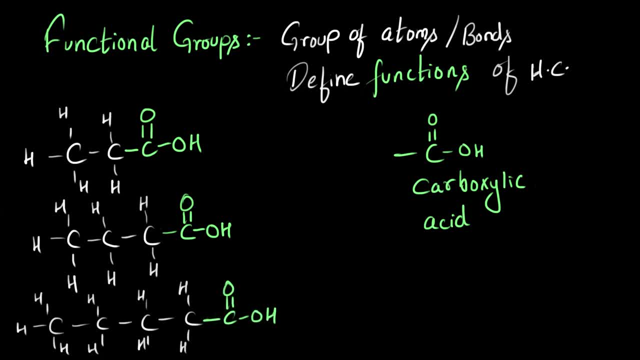 Here I have four carbon members. If I replace a hydrogen atom with this functional group, this molecule will also Start behaving like an acid and will have similar functions like all of these two. So all these three molecules have similar chemical functions, but they have different length of carbon atoms, The only 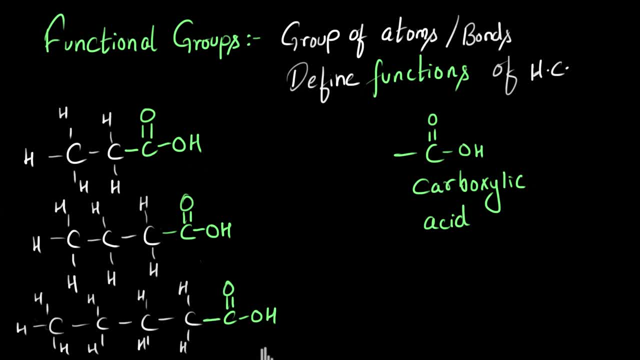 thing common is this group of atoms. So we can say that the common function, the common acidic function, is happening because of this group of atoms, right? So whenever this group of atom attaches to any hydrocarbon, it makes it have acidic functions. So in one sense we can say that. 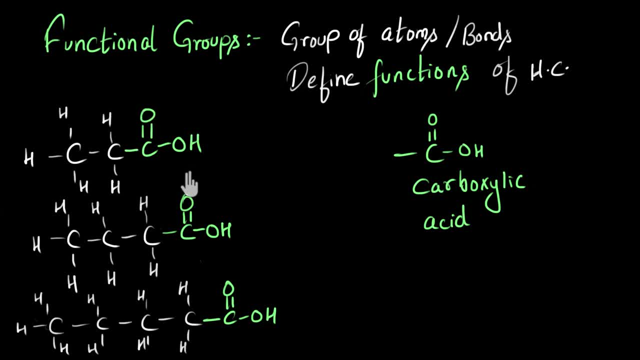 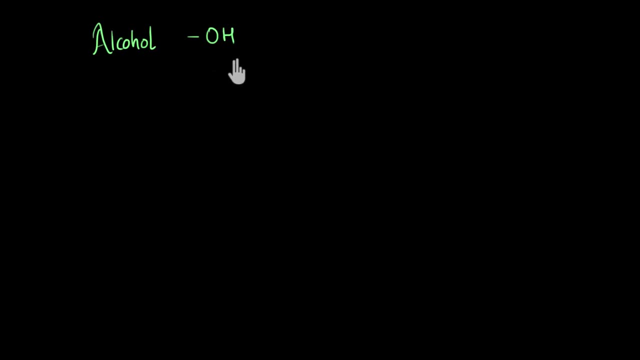 this group of atoms. it defines the function of the hydrocarbon right And therefore we call this group of atom a functional group. Now, with this, let's look at some other functional groups and their awesome functions that they give The group of atoms OH. they are called as alcohol functional group, So this: 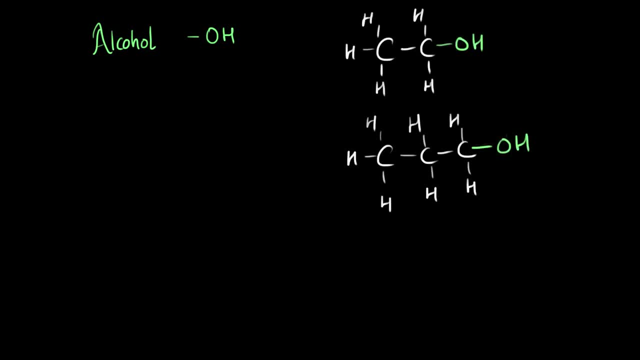 is how they attach with hydrocarbons, And when they do, they give them some special functions, For example, these alcohol molecules. they are all good antiseptics, They kill germs And they can also be used to dissolve various organic molecules. Now let's look at another functional group, The aldehyde group. 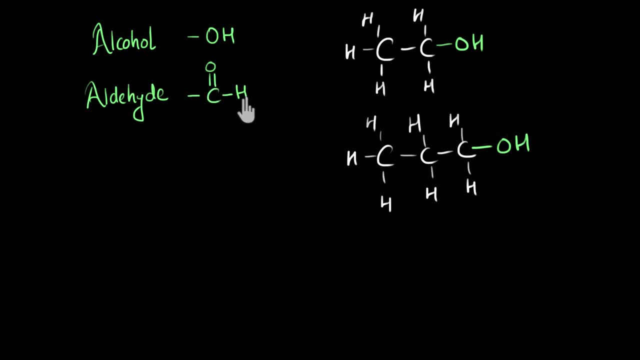 Here the group of atoms are C double bond with oxygen, And on one side it is attached with a hydrogen atom, So C double bond OH. Now let me show you how these group of atoms they attach with are hydrocarbons, Something like this: C double bond OH, and on one side there will be 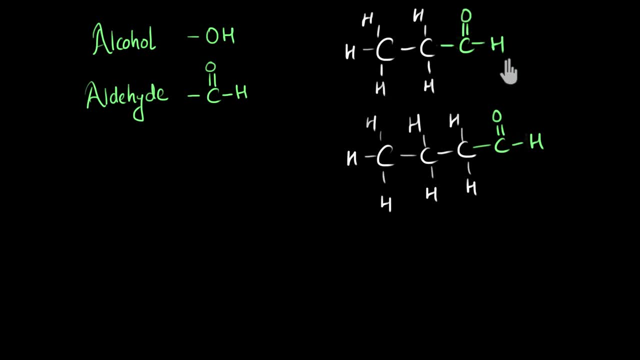 carbon chain. Okay, Now, when these group of atoms they attach with hydrocarbons, they give some unique, some special functions to them. That's why they are called functional groups, right. So the special function of aldehydes molecule is that they have a unique flavor And that's why they can be used in making. 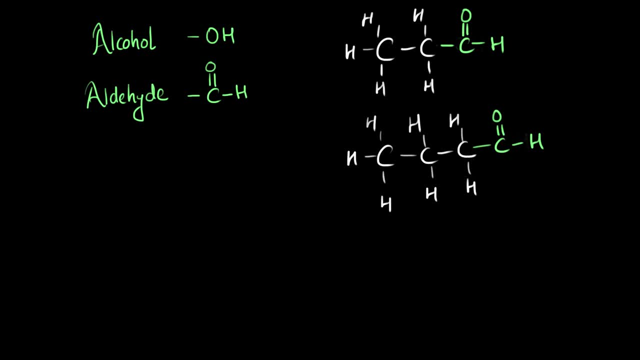 ice creams or some beverages. Now let's look at another functional group, The ketone group. The group of atoms over here are carbon double bonded with oxygen, And this is pretty similar to aldehyde. They both have a carbon double bonded with oxygen. 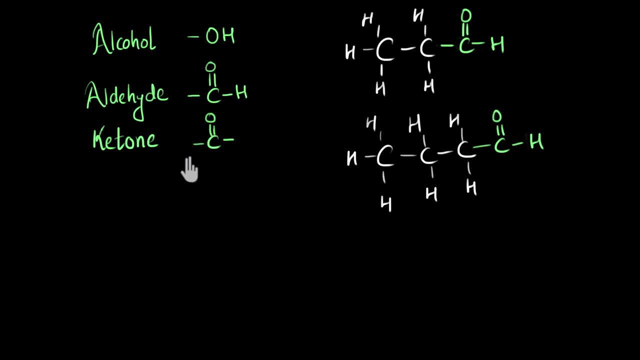 But the difference is that ketone is open at both ends. At both the ends we will have carbon chains attaching, Okay, Whereas in aldehyde, one side there is a hydrogen atom And only on the one side we will have carbon chains. So, for example, how ketone attaches with hydrocarbons is something like this: 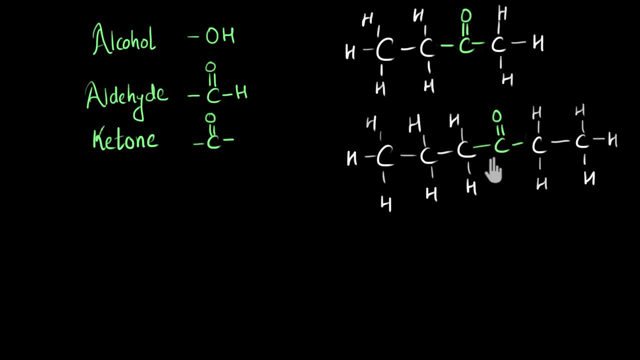 See C, double bond OH, And on both sides you have carbon chains. On both sides you have carbon chains. If one of these carbon chains were replaced by a hydrogen atom, Then we would be able to call this as an aldehyde group, Not as a ketone group. Okay, And now this has many special functions. 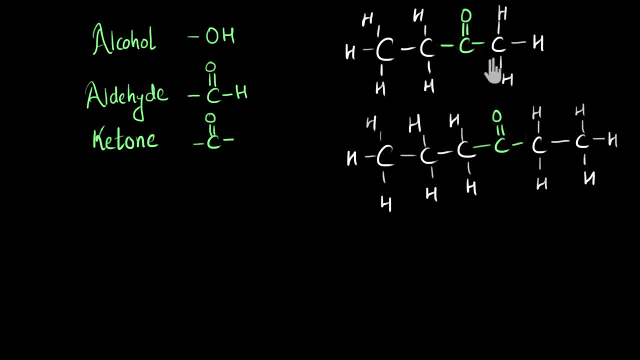 also Ketones. They are generally used in medicines. Okay, Now let's look at another functional group, The carboxylic acid. Well, we have already spoken a lot about them, But what I want to show you is that how similar these functional groups appear. See all of these three functional groups: Aldehyde. 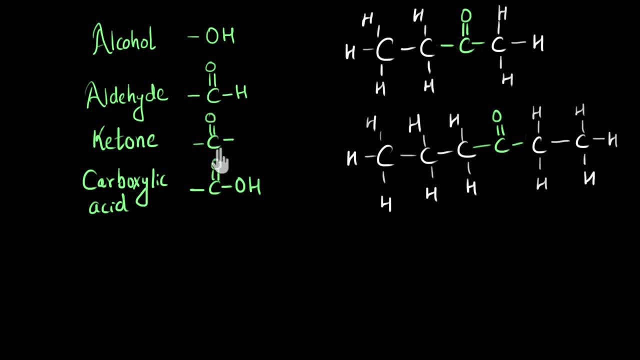 ketone and carboxylic acid. They have the C double bond O group in them, Whereas carboxylic acid and alcohol They both have the OH group in them, Right? So they might all appear very similar, But yet they are very different And they provide very different functions to the 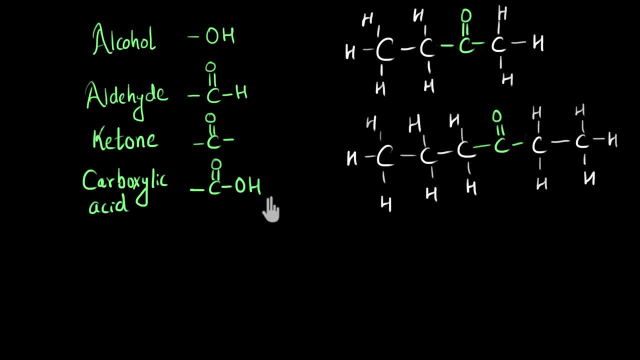 hydrocarbons that they get attached to. Okay, One more thing. All of these functional groups are commonly called as oxygen containing functional groups, Because you can see that all of them have oxygen atom in them Right Now. let's move on. Next, I want to talk about the halo group, The 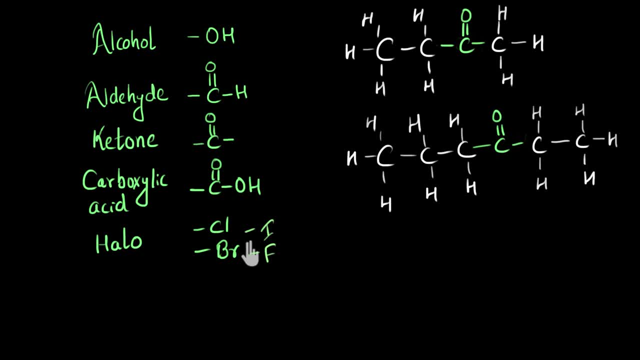 hydrocarbons, Basically the atoms of chlorine, bromine, iodine or fluorine. When they get attached to the hydrocarbons, They also impart special functions to them. They will appear something like this: See over here: This is a chloro group attached to the alkane family. This is a bromo. 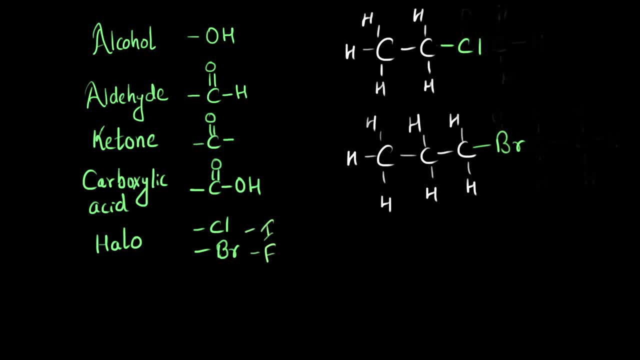 group attached to the alkane family. Okay, Now one last group, The double and the triple bond group. Yes, These are also functional groups. When they come in between an alkane, They provide special functions to the hydrocarbons. They also impart special functions to the hydrocarbons. They also 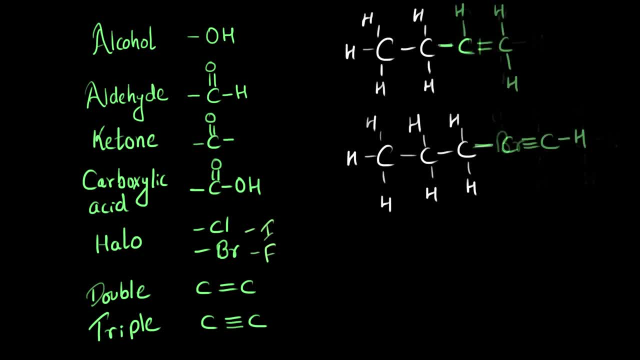 provide special functions to the alkane, And you might have already seen how they appear in the carbon chain, Something like this. So these are also functional groups. So we have seen a lot of functional groups And these are the broad categories. One is the oxygen containing: functional- 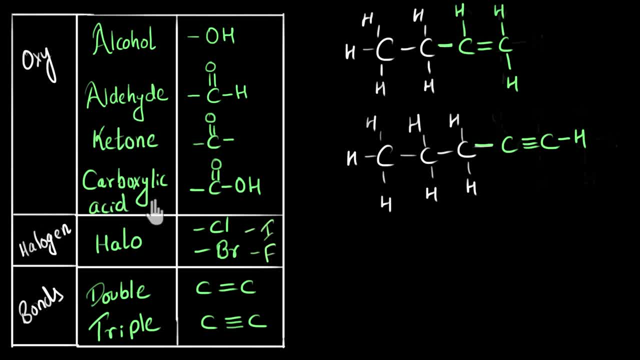 groups, Which has alcohol, aldehyde, ketone and carboxylic acid. The other is the halogen containing functional groups, Which include chlorine, bromine, iodine and fluorine. And the third category is of bonds, Double bond and triple bonds. These are also functional groups. 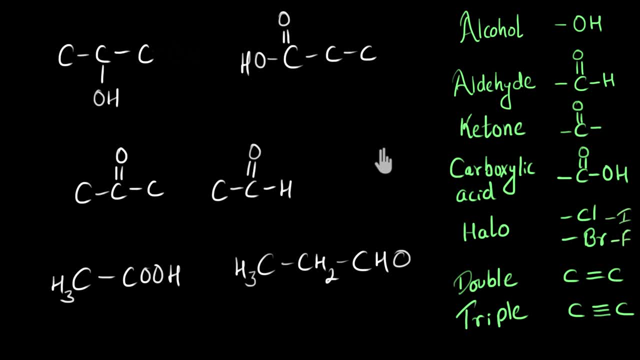 Now one last thing. On this screen you can see some carbon compounds, And all of them have some functional groups attached to them, And you might also notice that there are some carbon atoms which are missing, some hydrogen atoms, For example. this carbon atom can have three more hydrogens attached. 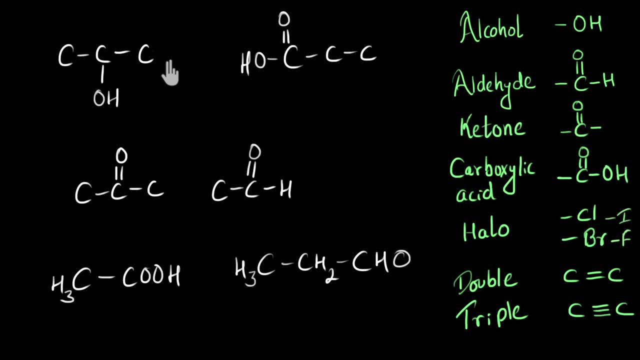 to it, But don't worry about them. I have not written the hydrogen atoms so that we can focus more on the functional groups. Okay, So over here I want you to pause the video and figure out which functional group is attached to which bond. So let's start with the functional groups. So let's 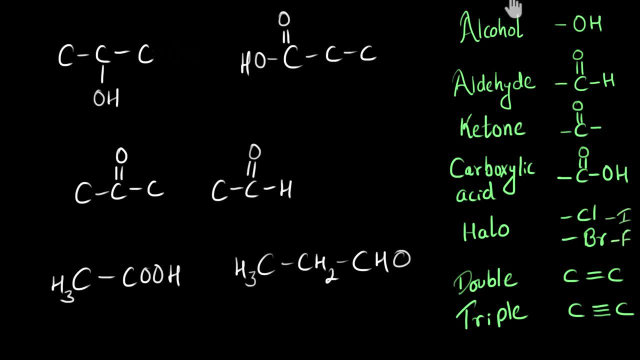 start with the molecule. For your reference, I have written all the functional groups and their names on the side, So pause the video and try it by yourself first. Now, if you have tried it, let's see. See over here in this one. 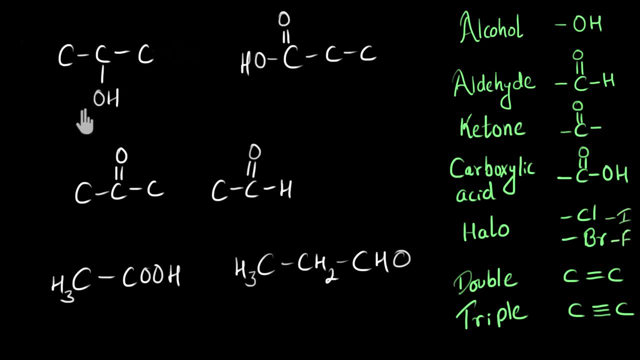 the first molecule. I see that this is the carbon chain and here OH group is attached to it, And OH group is called the alcohol functional group. So the name of this is going to be alcohol. Okay, Over here I see that this is the carbon chain and this carbon has double bond: oxygen and OH. 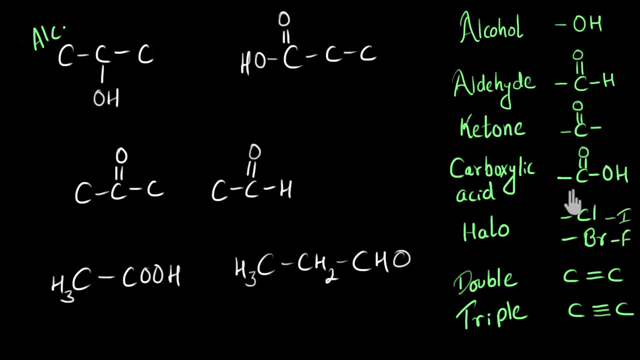 Now, if you look over here I can see that this functional group is what I notice over here: C double bond O OH. It doesn't look like arranged in the same order, See C double bond O OH on the right, but here OH is on the left, But that doesn't matter, Right? So this is the carboxylic acid. 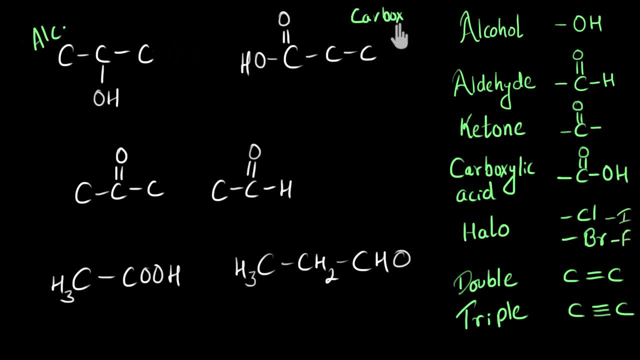 functional group- Carboxylic acid functional group. Okay, Now let's look at this. Here there's a carbon chain. This carbon has double bond O attached to it And on both side it's attached to a carbon atom. So that you can see, over here in the ketone, Over here C double bond O. 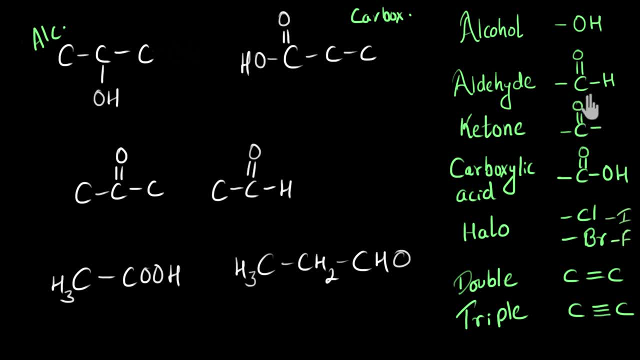 and both sides are free to be attached with carbon atoms, not aldehyde. See, aldehyde has one hydrogen atom on one side. Okay, So this is going to be ketone. Similarly over here. if you look, this carbon atom is double bonded with oxygen And on one side there is an hydrogen. Okay, Only one side. 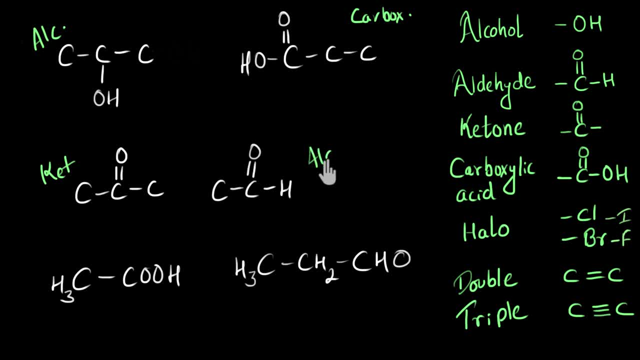 it is attached with a carbon, So this is going to be an aldehyde, not a ketone. Now let's look at this one. So this is strangely written here. I do not see the structure of the molecule, but I have the molecular formula. but see, I can notice that this part has oxygen in it, So this is going to be. 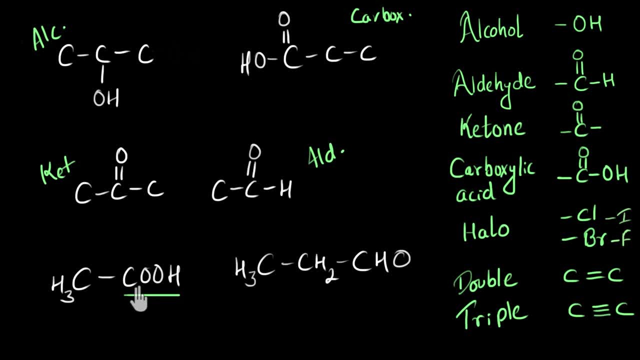 the functional group. Now this has two oxygen: C, double bond, COOH. Okay, And there is only one functional group with two oxygens. this one carboxylic acid. So this is going to be our carboxylic acid functional group. Now the last example in this molecule: 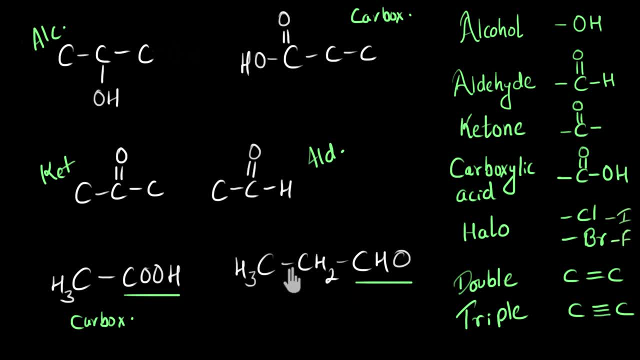 this is going to be our functional group because it has oxygen. See, this is the carbon chain and this is our functional group. Now, which functional group is this? Is this the alcohol? Because alcohol has OH, and this one also has OH. But see, if alcohol were the functional group, it should be.